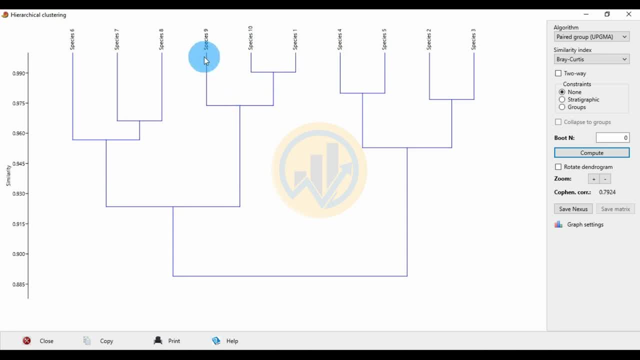 the species 1 and the 102 the similarity there were. the next one group for the species 9 and the species 8 and the species inch For the speciespecies squaredWE кол那我們. Utme device tests in d europe. verboxist đây. 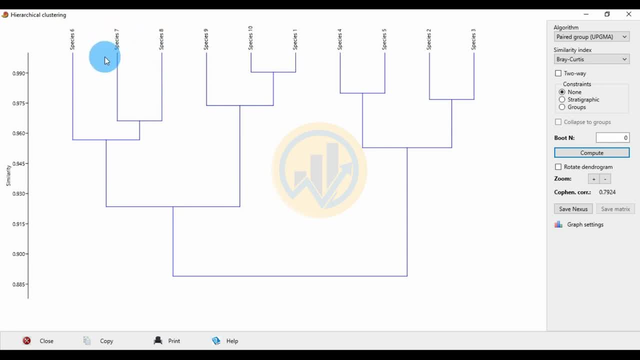 Species 8 and species are also the first group for the similarity and species 6 equal to the similarity for the species 7 and the species 8.. Now the comparison for the 10 species and to the morphometric parameter of the species. Before we click the checkbox for the two way method, click the checkbox and click the computing. 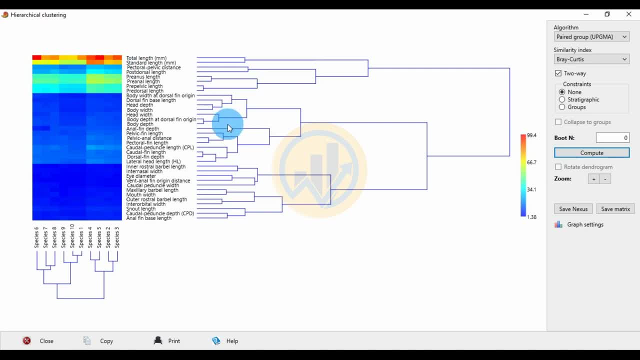 button. This is a two way cluster analysis for the three species Before the morphometric parameter: the analysis for the clustering, the first group for the most of the first group, presenting the second group for the. this is a second group. this 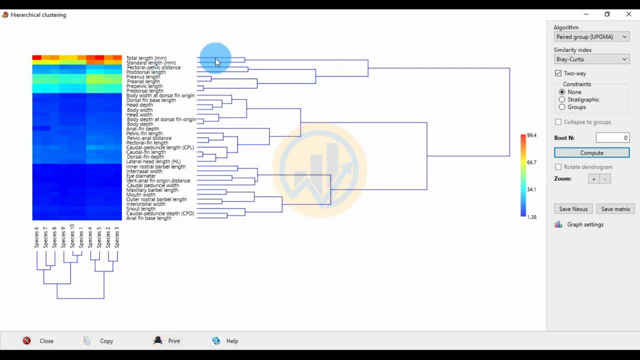 is a third group. this is a fourth group. The first group, very similarity for the total length for the three species and the standard length. also the first group, the highly similarities. The next one, the group for the similarity in the postal pelvic distance and the postal. 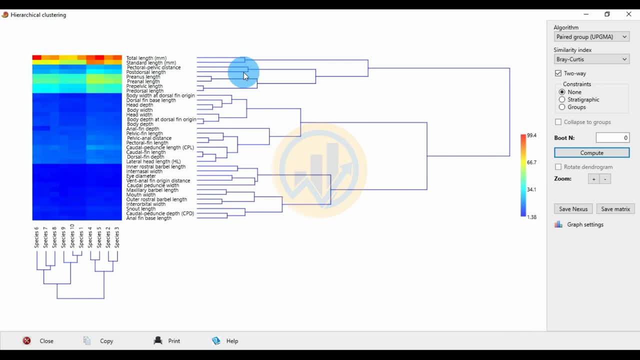 length. also the second. first group for the similarity, This group also similarity for the second and the third. for the first group, the first group and second. this is a first group for the compare similarity to a second and third group. this is a fourth group. 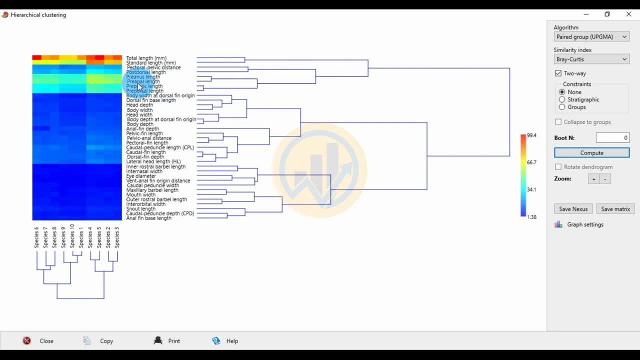 The next one for the pre-anus length and pre anal length. also the third, first group for the similarity At also the same time Pelvic length and dorsal length. also the similarity: this group was a single group. This first group, primary group, compared for the secondary group, Then this pelvic length and pre dorsal length. also the similarity for the second group in the pre anal length and pre anus length. 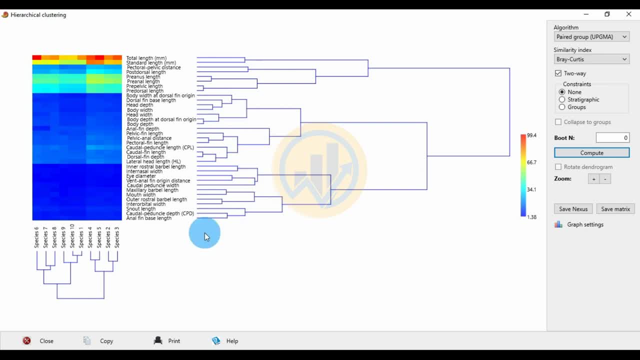 This is for the marbometric comparisons and next one for the same for the species comparison for the species 3 and 2. so the similarity for the first group and species 5 and 4. also the similarity in the first group. This also species 1 and 10, also the first group. The second group for the species compared for the species 9, species 10 and species 1.. This color also indicated for the two way clustering. 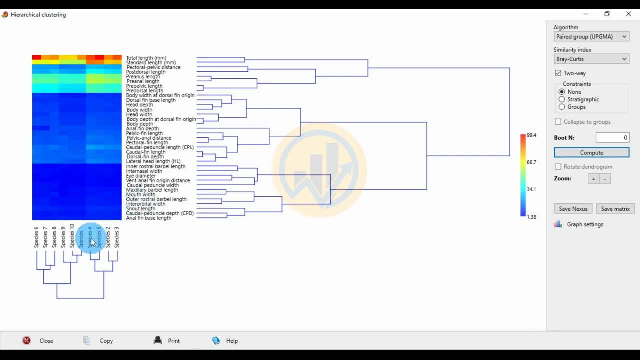 analysis in the swiss pcs. the morbo metric and the swiss pcs. the highest range for the blue color, for the 1.38. the similarity and very distant similarity for the highest in the red color in the 99.4 for the red color. this is for the graph for the clustering analysis in the 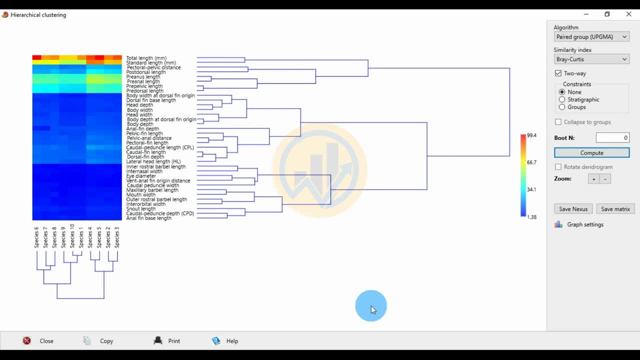 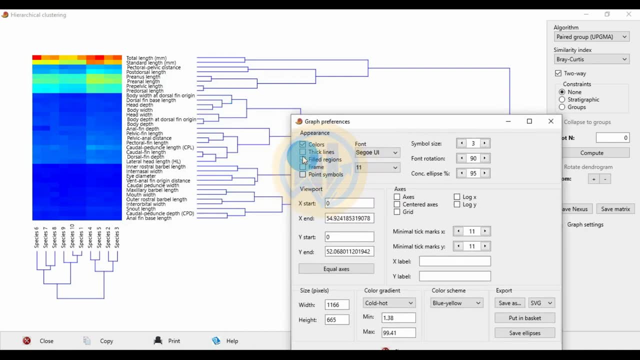 swiss pcs, the two-way clustering analysis. now the change the graph. the go to the crop setting the before the want the check thickness for the lines. they click the thickness lines and change the font for the stay. now the change font. we know. now we change to our time, roman. 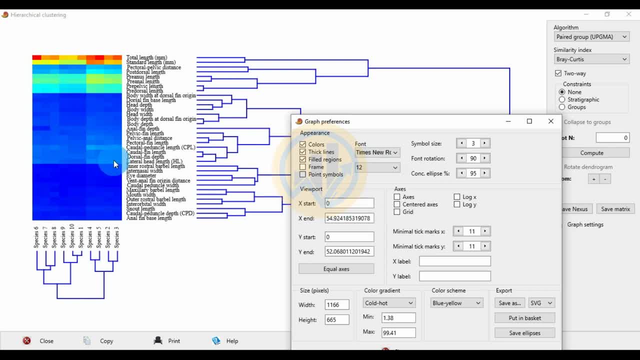 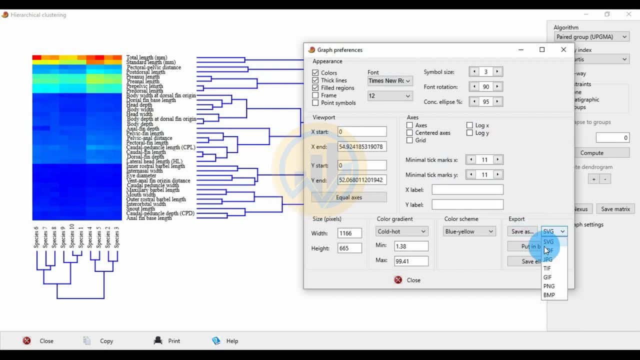 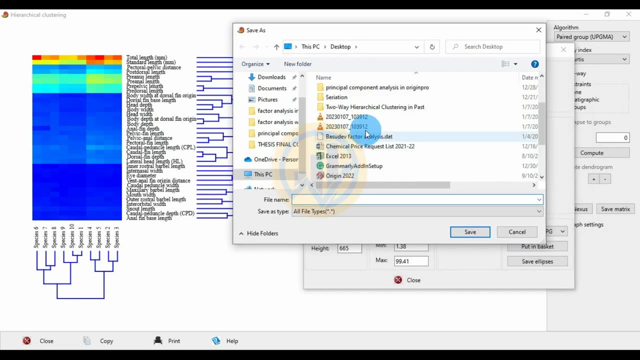 select the time roman and the font size is 12. change the font size is 12.. ok, now the seven. the graph for the export. the change the format for the jpg. okay, click the save as button. okay, now the change the save the graph for the. enter the name. 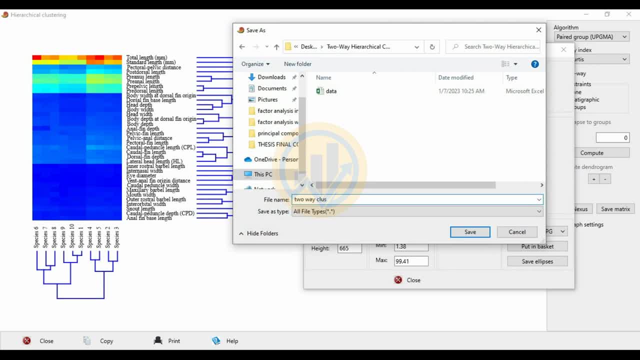 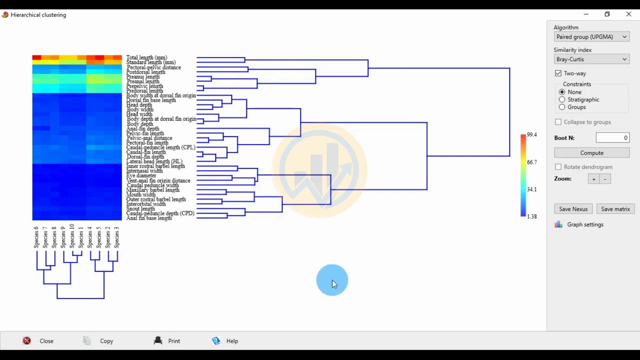 two-way clustering. okay, save it then close it. thank you for watching this video. if you like our channel video, please subscribe and join the membership. thank you again.